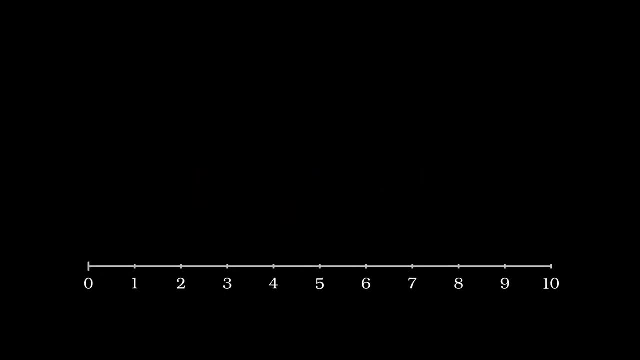 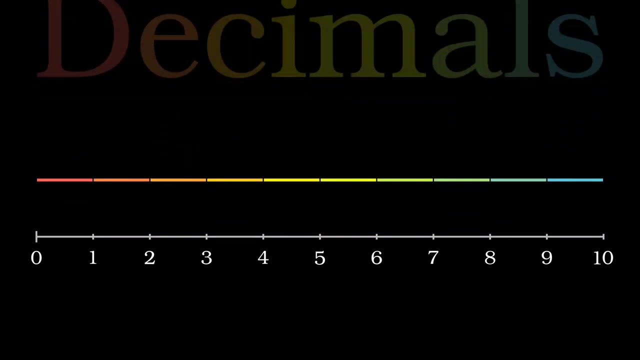 than three. In this case, we are looking for some new numerical entities in between our everyday natural numbers. Luckily, we don't have to work too hard to pick some of them, as these colourful segments are seething with numbers, also known as decimals Now each. 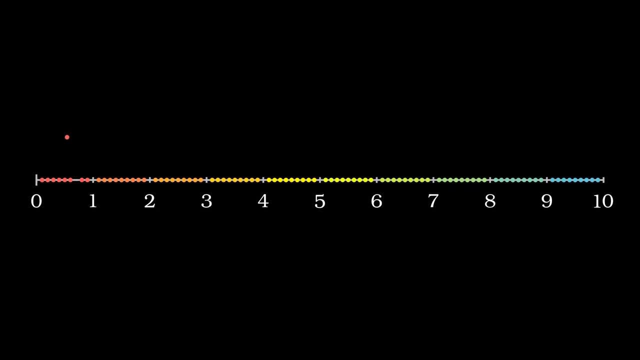 of these colourful dots between whole numbers represents a decimal. So even though we don't know exactly the decimal that this dot represents, we know for sure that this mystery number is greater than zero, but smaller than one. Similarly, we deduce the inequalities for other decimals on the number line. 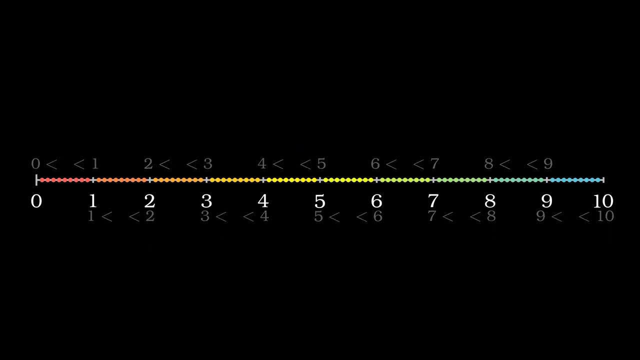 Now let's put all these dots back where they belong. The truth is that, while whole numbers can be found only at specific points on our number line, decimals can be found practically anywhere in between. And although our number line seems to be packed with decimals represented, 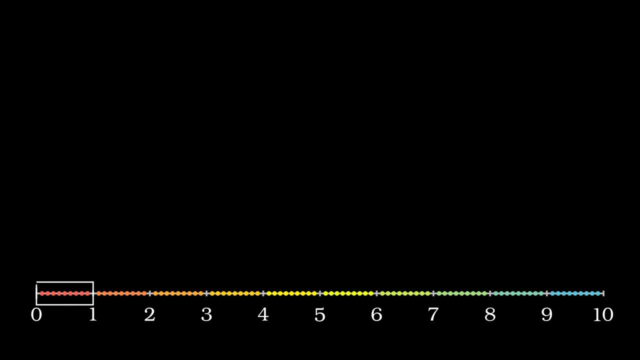 as colourful dots. if we take a closer look, we will notice that there is still some room for more dots, meaning more decimals can be found between any two decimals, regardless of how close they are. The more we zoom in, more and more decimals will come into visibility. 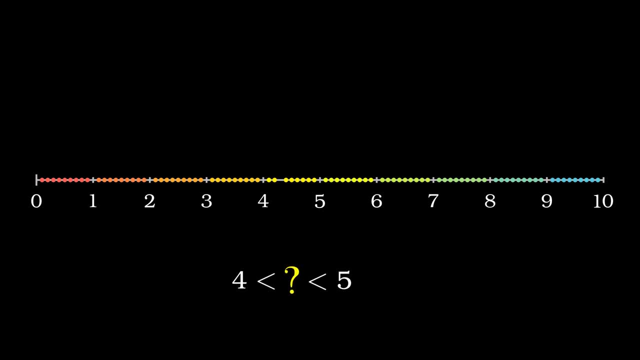 Now the question is how decimals look like as numbers. what kind of digits should we use, and in what order? If we used numerals, this dot would be exactly 4.3.. But why, Well, the first digit number? 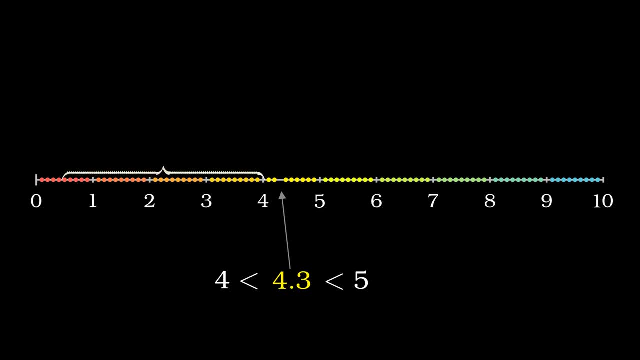 four is the whole part that we are familiar with, But the second digit, number three, shows how far from number four are decimals still present. Here we can see that, the number. To understand that fractional part of our number, as we call it, we need to see in more detail how small it really is. 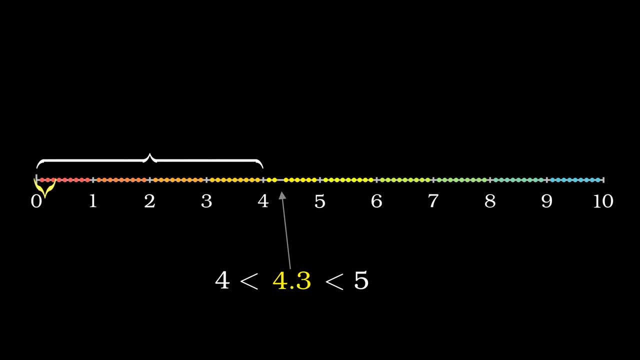 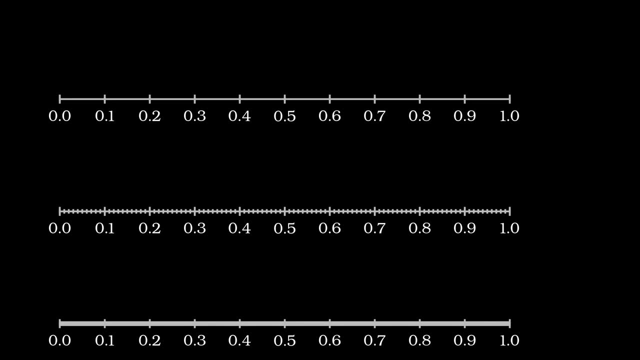 So let's take a closer look in the neighborhood of zero. Here we have three identical number lines divided into line segments of equal length. The third number line also contains segments, but they are too close to each other to be visible. But if we zoom in we can clearly notice the small gaps in between. 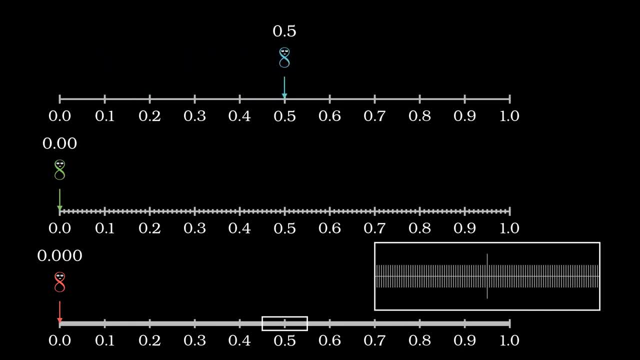 As we scan the number line, the number that appears after the decimal point is exactly the number of the segments covered at that time in each line. The only difference is that in the first line we keep counting more numbers, but in the end all the creatures stand right in the middle of the exact same line, that is, they have arrived at the same number. 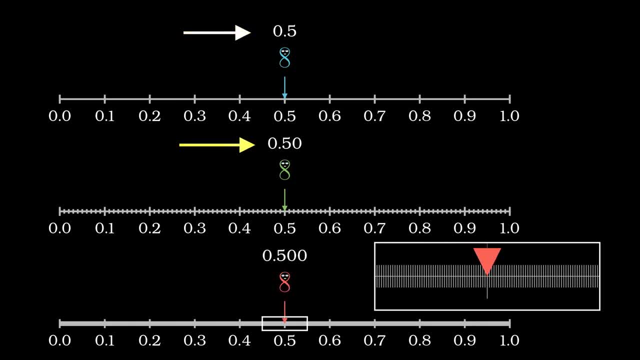 That's why 0.5, 0.50 or 0.500 is the exact same number. 0.5, 0.50 or 0.500 is the exact same number. 0.5, 0.50 or 0.500 is the exact same number. 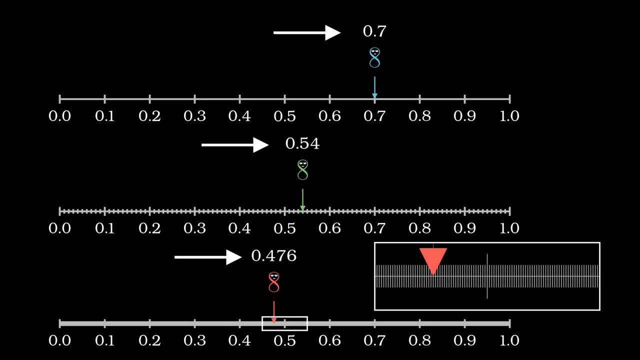 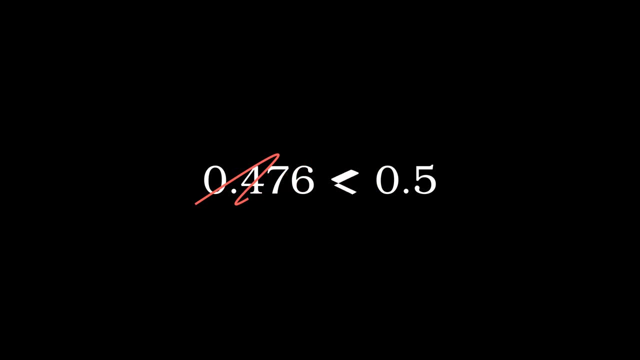 Now let's have a look at these three numbers. The number at the bottom of the screen is the smallest of all three, as its distance from zero is the shortest. So the fact that a decimal has more digits on the right of the decimal point doesn't mean that it's necessarily greater than a decimal with fewer digits in its fractional part. 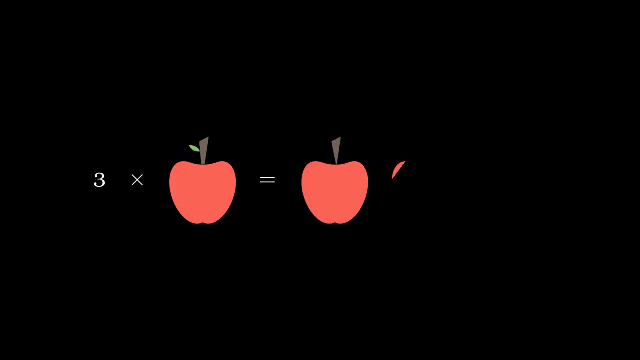 Just like natural numbers, tell us how many whole objects let's say exist. Just like natural numbers, tell us how many whole objects let's say exist. just like natural numbers, tell us how many whole objects let's say exist. use the maximum number of words we have in total. decimals can show how much of an object or a quantity we have. 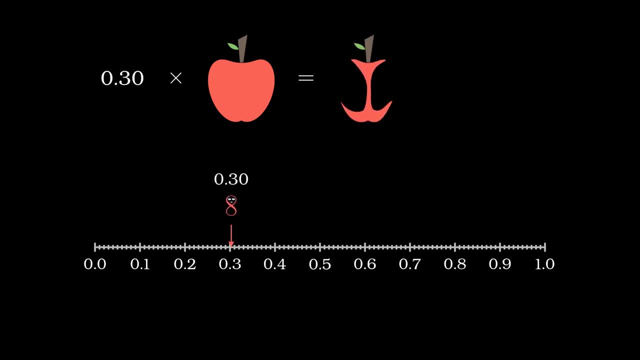 In this example we explore how the total amount of quantity changes as we multiply it with numbers smaller than one. So here we have an apple, or what's left of it, approximately according to the decimal number we use to express that quantity in this rather unusual equality. 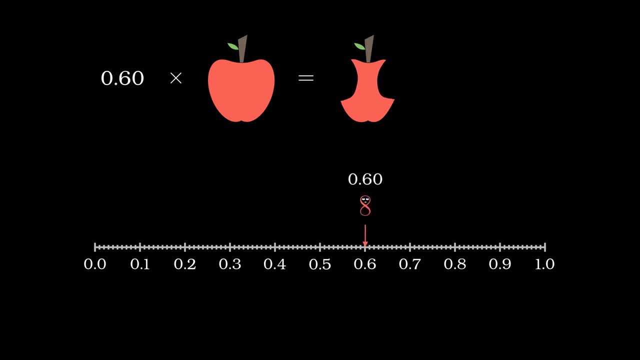 From nothing, that is, 0, or almost nothing. when we are close to 0, to a whole apple and anything in between one, the closer we get to enjoy a whole apple. It seems that whole numbers don't tell us the whole story. 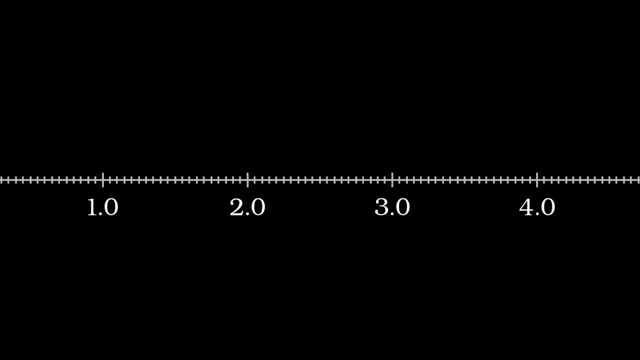 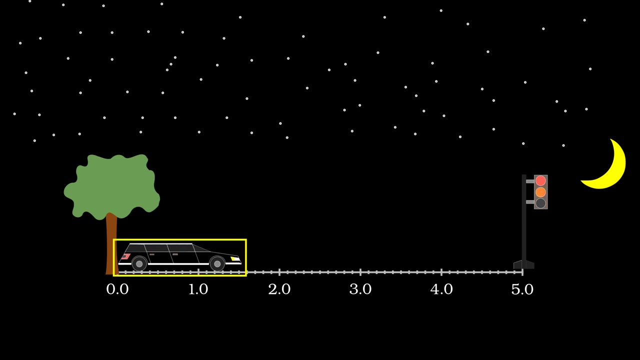 We need more and more numbers- the numbers in between- to fill the gaps in our narrative and understanding, so that we can better and more accurately describe the world around us and everything in it like objects from our daily lives, Just like this car. we've got right here and some details about our little trip with 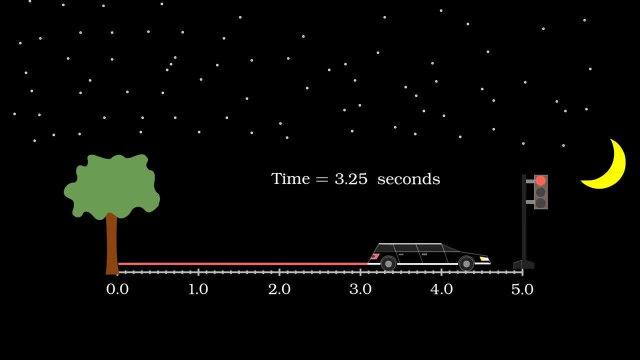 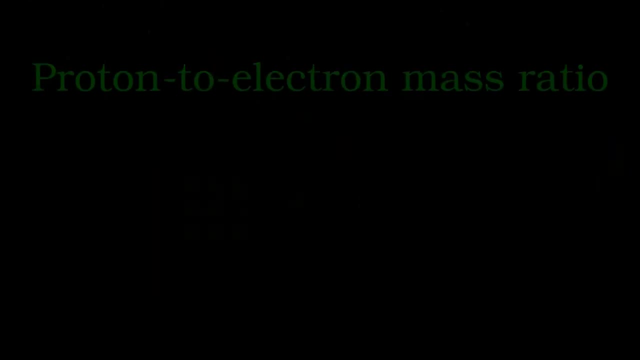 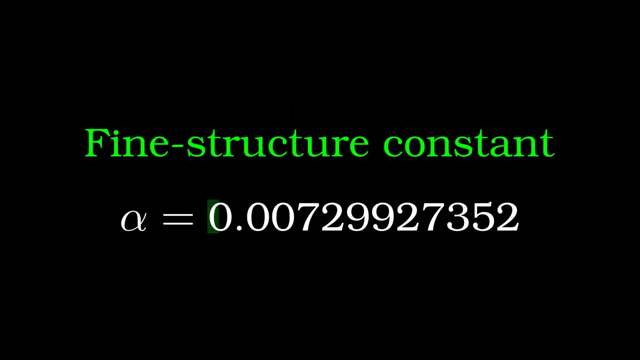 it that we can actually measure, From the time elapsed, distance travelled, average speed, everyday heights and widths to cosmic distances and, of course, universal numbers, also known as physical constants that appear in nature uniquely characterising the universe we live in.